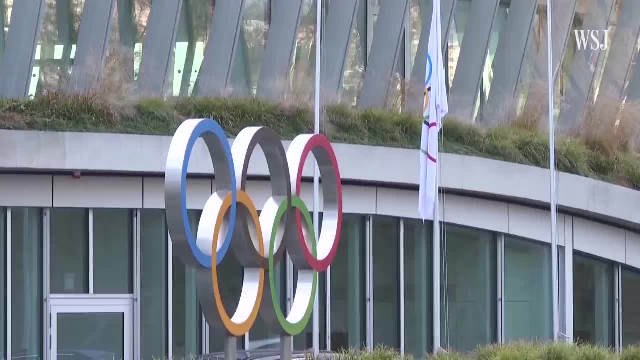 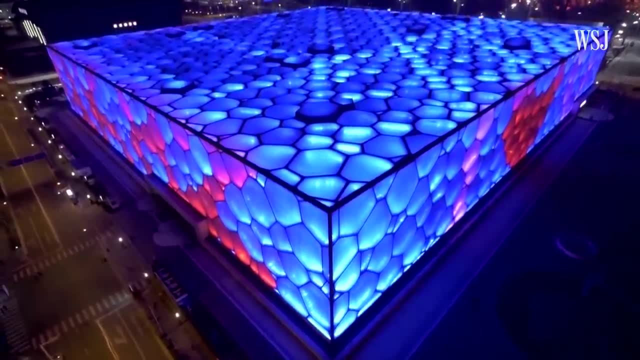 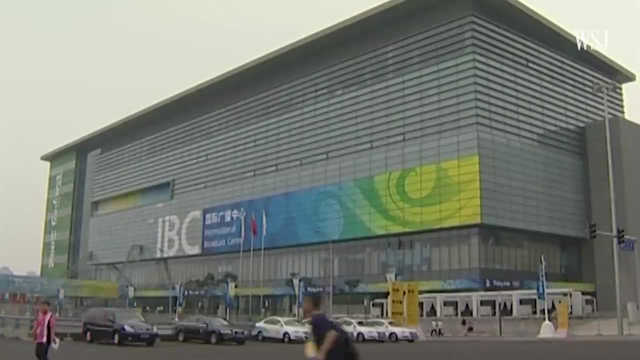 75% of the IOC's total income. This year, the Beijing Olympics is being broadcast in more than 220 countries. China Media Group is airing the games in China, Discovery is airing it across Europe and CBC is airing it in Canada. Since 1997, North American companies have 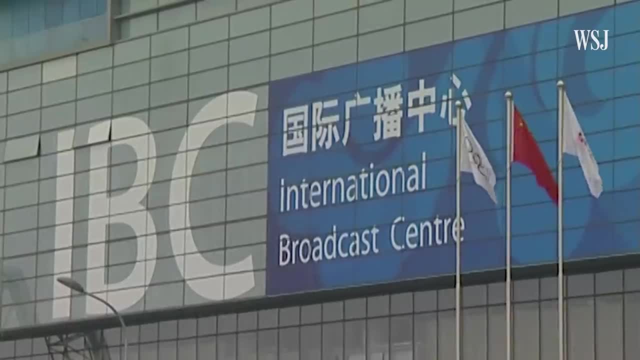 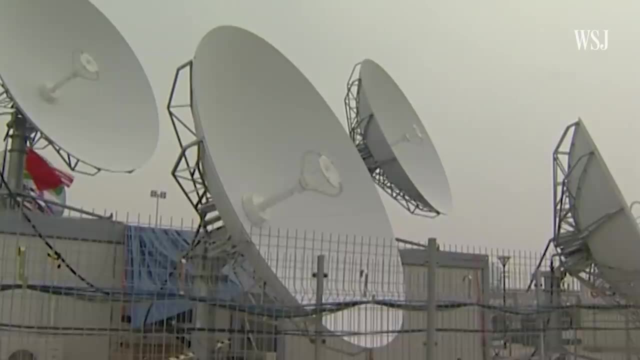 paid more for broadcast rights than the rest of the world combined, according to IOC data, And NBC has televised every Olympics since 2000,. and every Summer Games since 1988. I've come to associate NBC as being the channel of the Olympics. 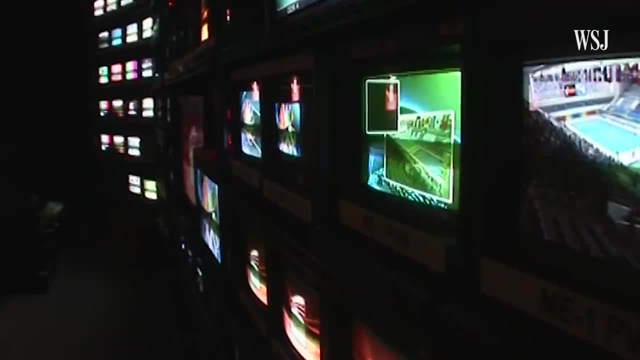 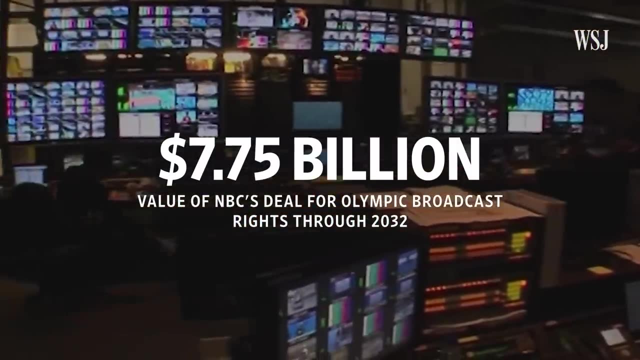 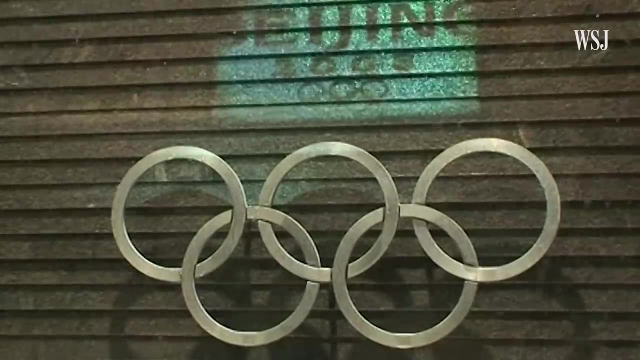 and I'm sure many other Americans do so as well. In 2014,, NBC entered into a $7.75 billion deal to secure exclusive broadcast rights in the US through 2032. That means the company will pay an average of over $1 billion for each Olympics. The deal covers all media platforms, including 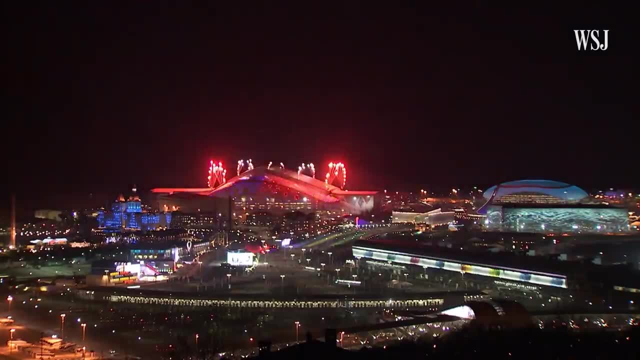 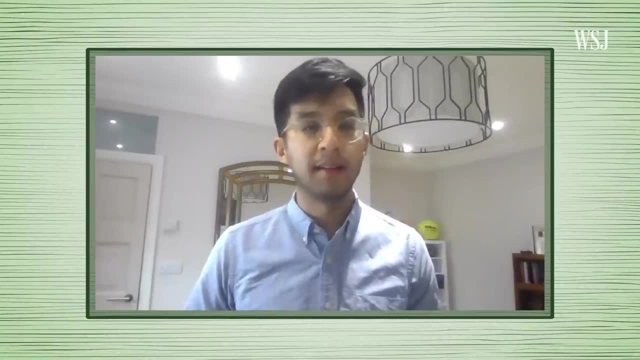 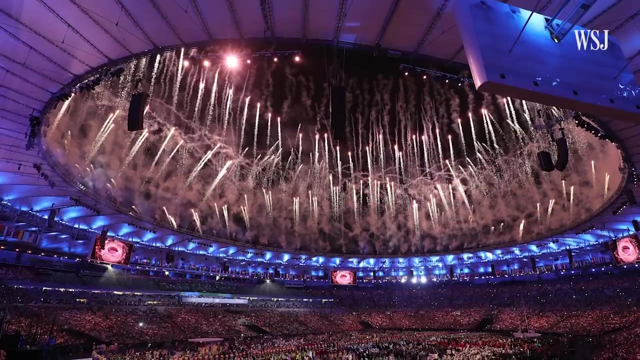 TV, internet and mobile rights, and also restricts other media from broadcasting the opening and closing ceremonies and athletic competitions. When it comes down to getting these broadcasting rights, it comes down to one thing, which is money. These multi-year broadcast deals include both Summer and Winter Olympics, For example NBC. 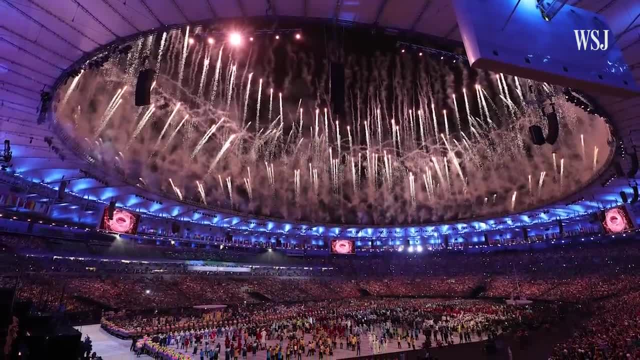 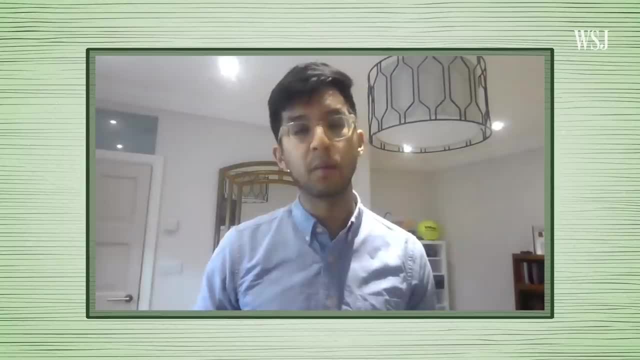 Universal made about half a billion dollars more in revenue from the 2016 Summer Olympics than it did from the 2014 Winter Olympics. according to the company's financial statements, The Summer Games are a lot bigger than the Winter Olympics. There's about 200 countries that compete in the Summer Games. 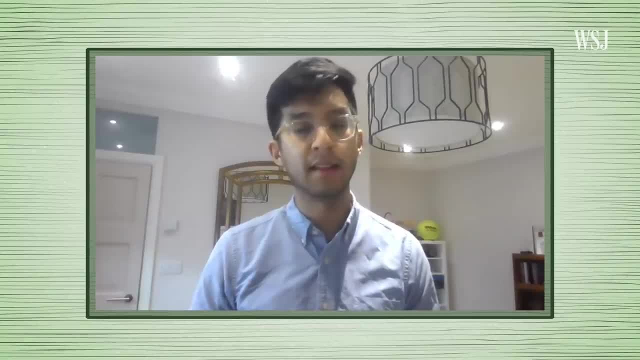 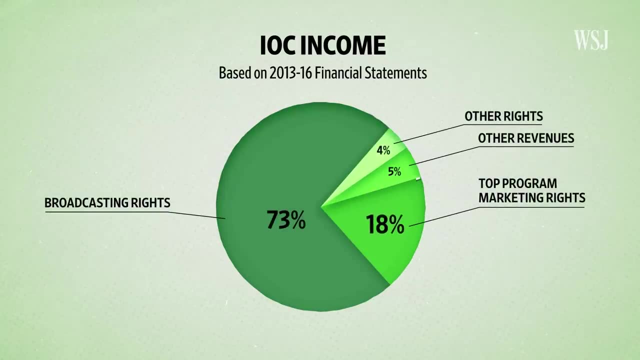 about only 100 in the Winter Games. There's a quarter of the athletes in the Winter Olympics compared with the Summer ones. After broadcasting rights, brand partnerships are the next income driver for the IOC, The Olympic Partner Program, which was launched in 1985,. 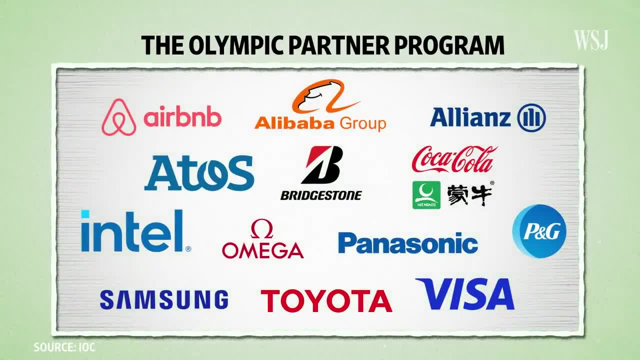 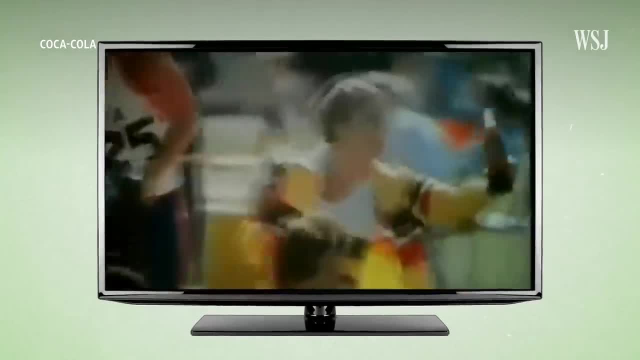 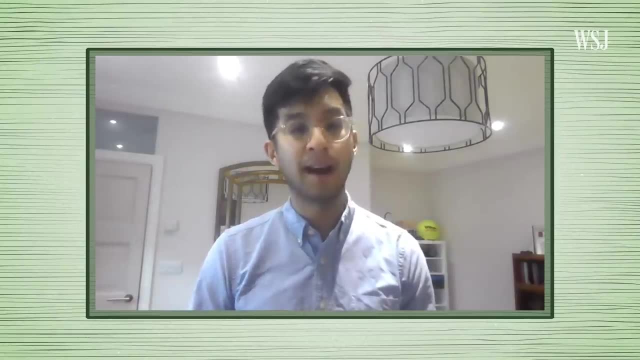 grants exclusive marketing rights to a select group of corporate sponsors. There are currently 13 top-tier sponsors in this program, So you have companies like Coca-Cola been around forever, But you also now have tech companies like Airbnb and Alibaba in China, who have signed up in the past decade for these multi-year deals to be one of the elite sponsors. Alibaba believes in the power of small. We are proud to be the worldwide partner of the Olympic Games. According to the latest IOC data, top-tier sponsors collectively paid around $1 billion for the 2014 and 2016 Olympics, And that's a lot of money. 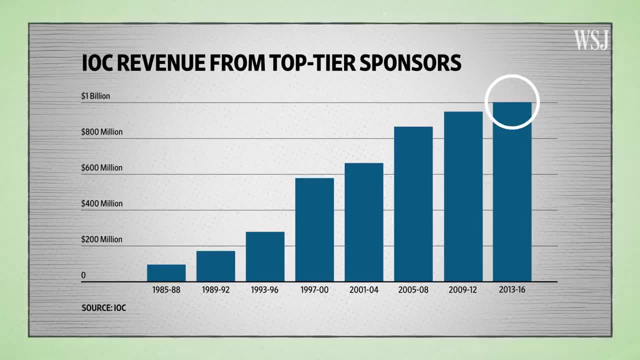 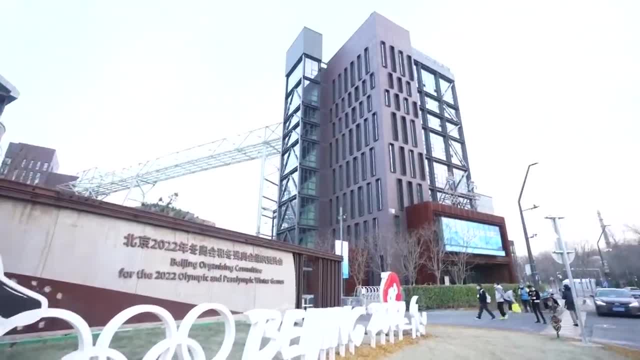 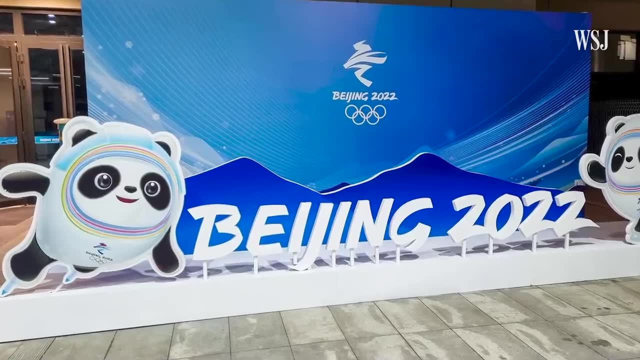 And that's a lot of money. So what do these brands get in return? They get to use Olympic logos. So the iconic rings, the five interlaced rings, are probably the best example, But also there's an official logo for the Beijing Games and the Tokyo Games, and all that too. 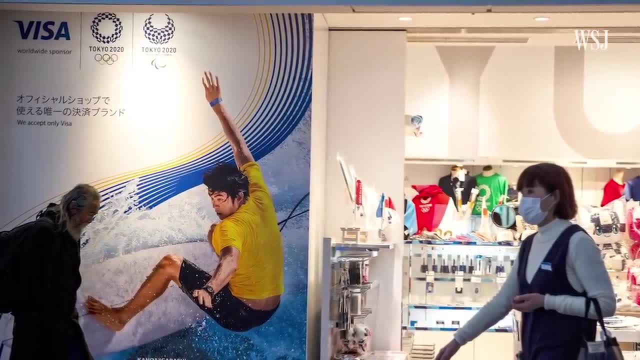 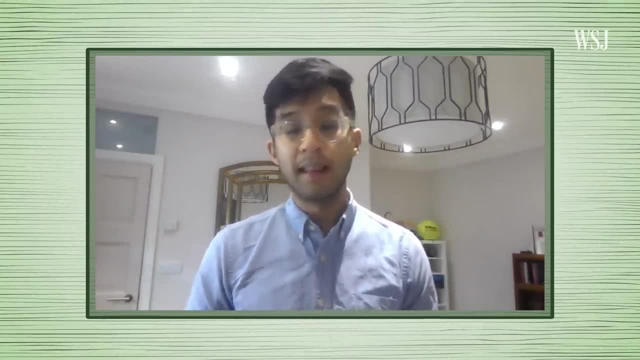 But buying sponsorship rights is just the first step. They spent a lot of money- tens of millions of dollars- per Olympics just to get the rights to use these Olympic logos. And then they got to spend even more money- maybe triple that- to tell everybody that they have these rights. 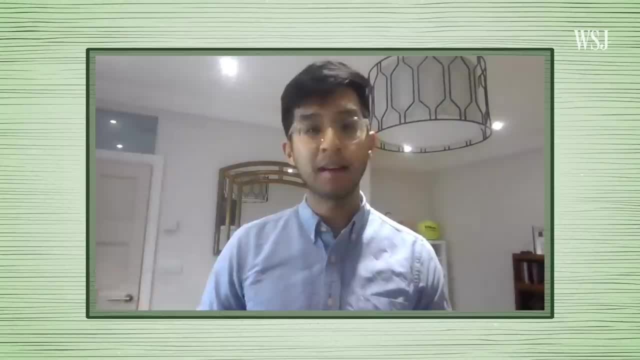 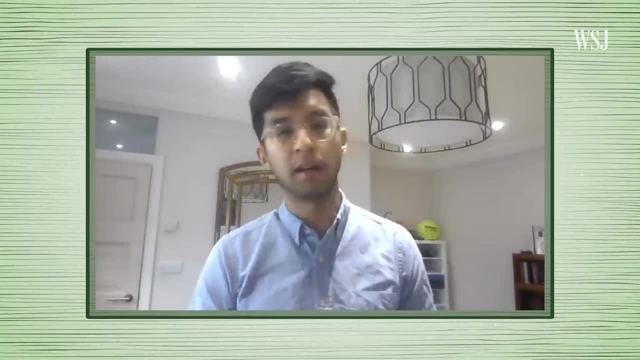 via TV advertisements that say: hey look, we're helping to put up these feel-good games that brings the world together. Or if you're Coca-Cola, they might want an athlete to go around drinking a Coke at the Olympics, And it also costs money just to put the rings on a can or a bottle of Coke. 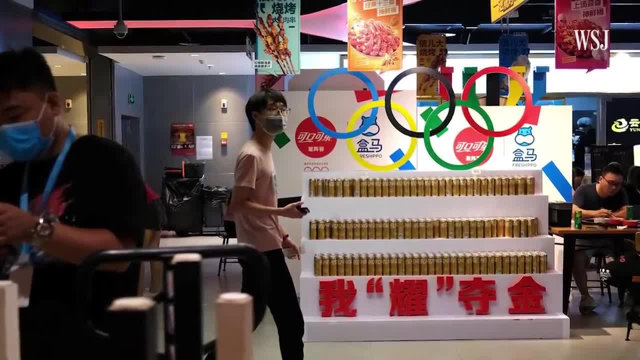 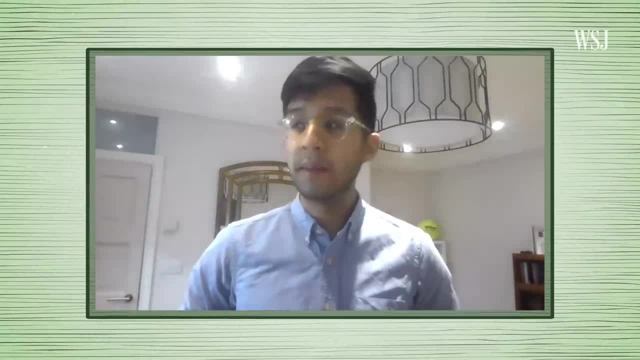 These brand partnerships are multi-year deals, often spanning four or five Olympics, which means the IOC doesn't have to scramble to find a new sponsor every two years. Airbnb, just a couple of years ago, signed a 10-year deal, So that'll take them through the. 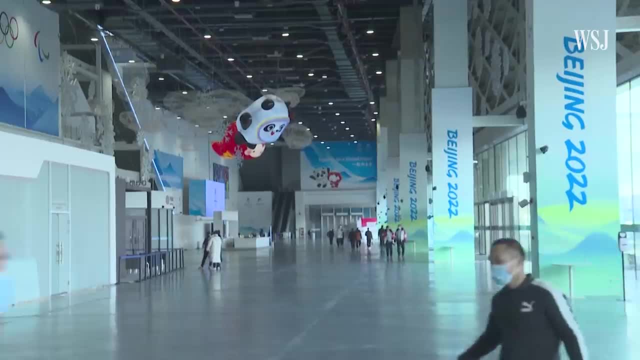 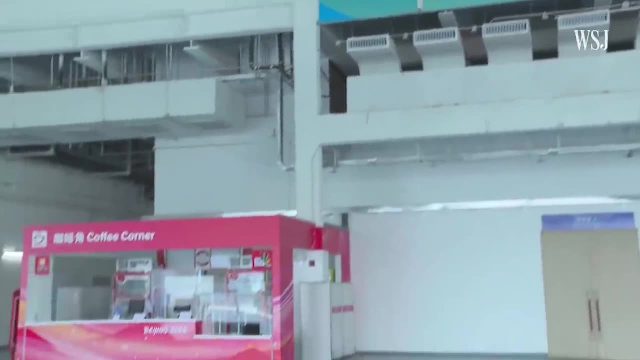 2028 Olympics in Los Angeles. This year, several Olympic sponsors are keeping a relatively low profile around the Winter Games in Beijing due to escalating tensions between the US and China. In a normal Olympic year, these companies that already spent a lot of money. 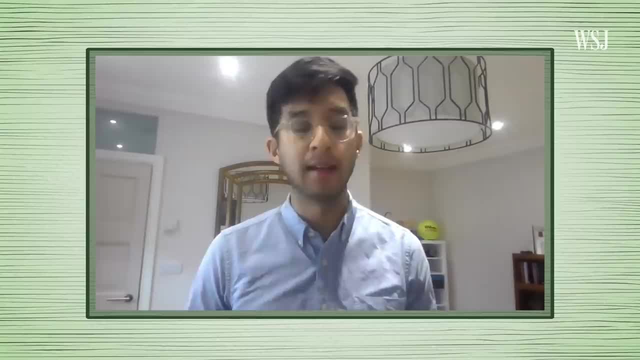 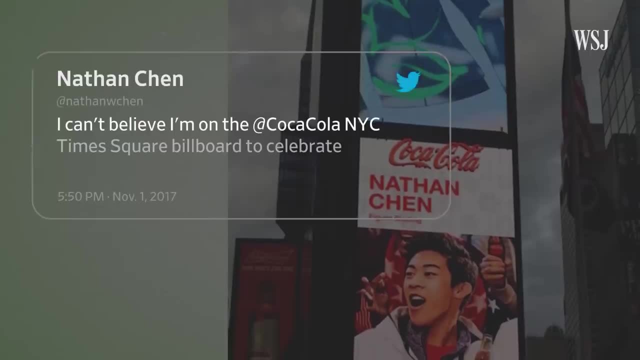 to be a top Olympic sponsor would normally be bragging about it. The 100-day countdown is usually a big thing. For example, ahead of the 2018 Games, Coca-Cola put figure skating star Nathan Chen on a billboard in Times Square to mark the 100-day countdown. 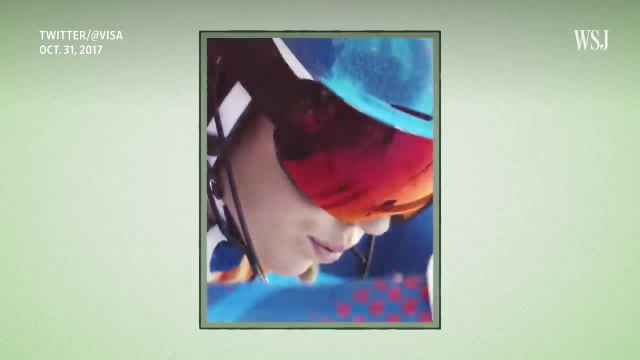 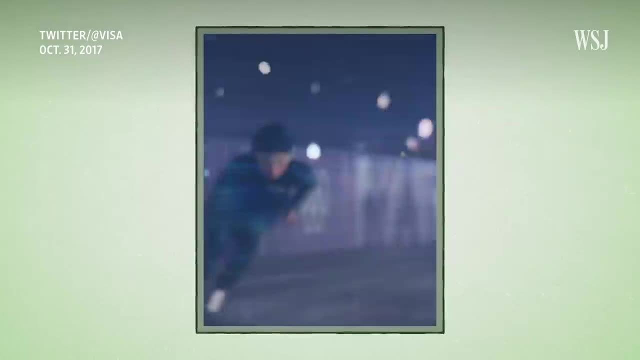 And Visa, which sponsors athletes through its Team Visa program, tweeted about its athletes and promoted its wearable payment devices in the weeks leading up to the 2018 Games. You dream of amazing. We dream of amazing ways to pay. Companies make million-dollar investments in these sponsorship deals. 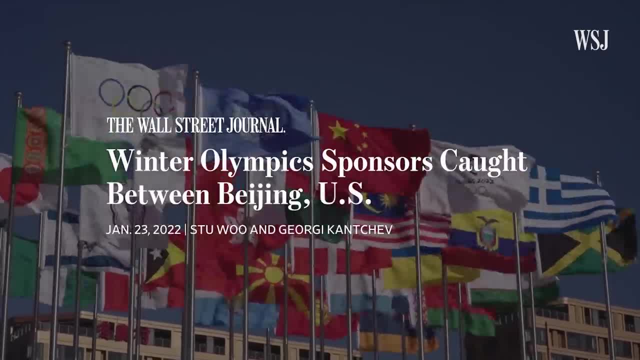 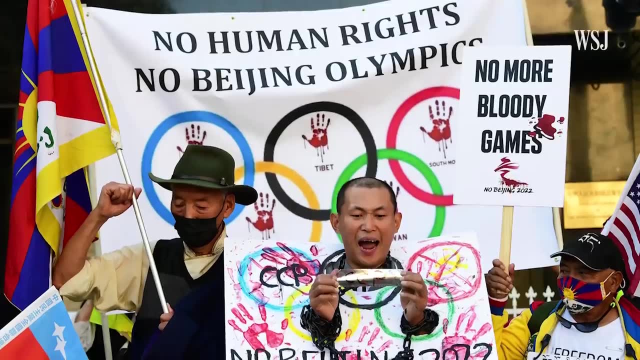 But this year sponsors may risk missing global marketing opportunities. that money bought them. US officials, some Western lawmakers and human rights activists have said Beijing's years-long campaign of global marketing a forcible assimilation against the mostly Muslim minorities in Xinjiang.